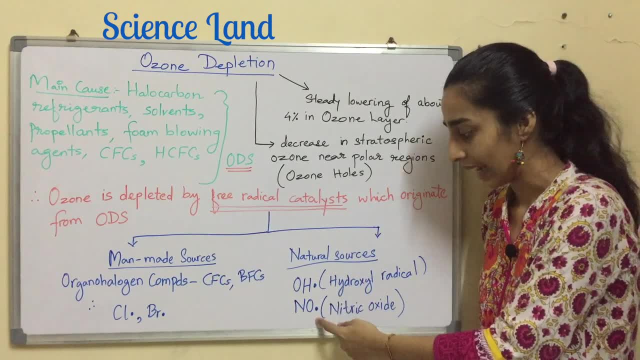 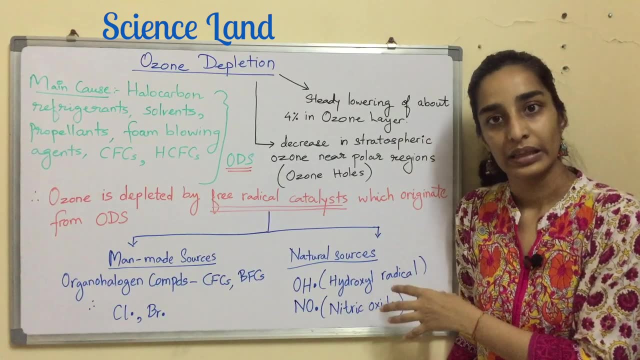 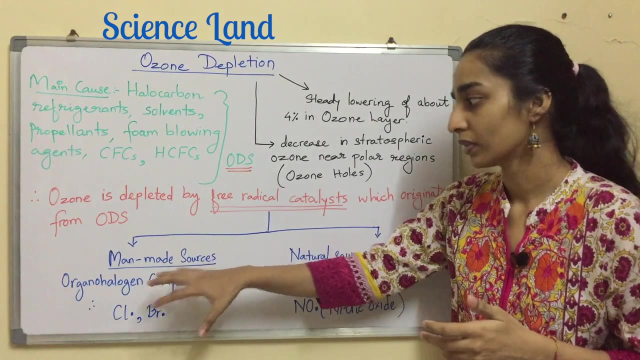 sources So radical like OH NO. OH is the hydroxyl, radical, NO is the nitric oxide. These radicals are naturally there in the stratosphere. That's the reason. natural sources, Man-made sources, are basically organohalogen compounds, which are CFCs. 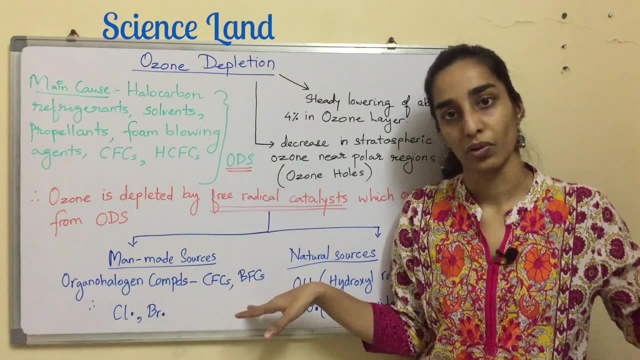 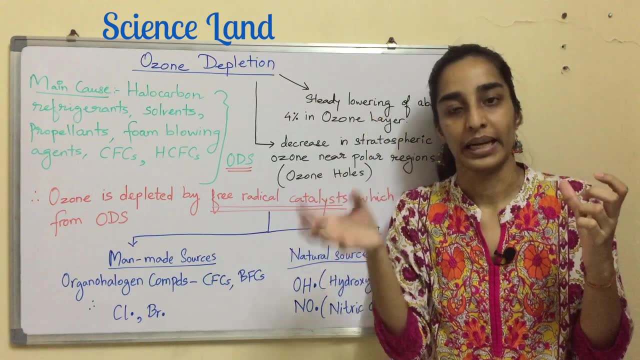 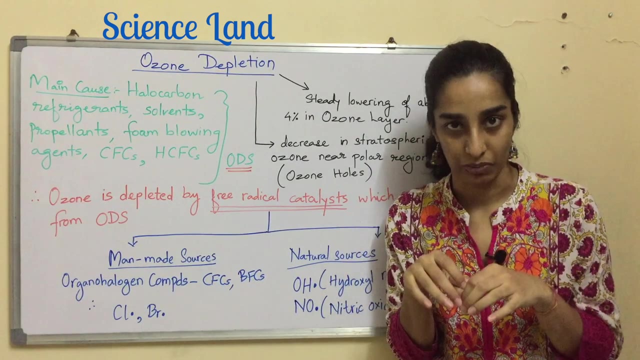 Chlorofluorocarbon, bromofluorocarbon. If you don't know, organohalogen, as in the organic part, is there and at the same time, halogen, which is chlorine bromine. all these halogens are there in the compound. That's the reason, organohalogen compound. Now the mechanism. 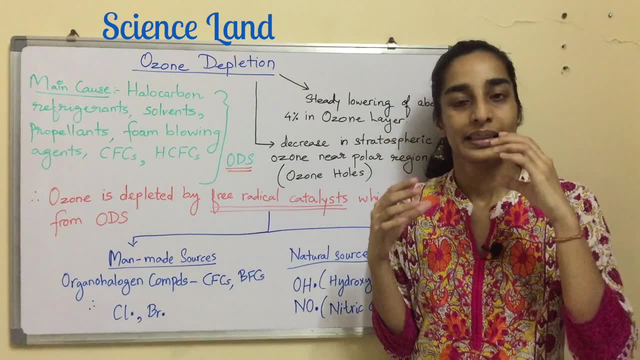 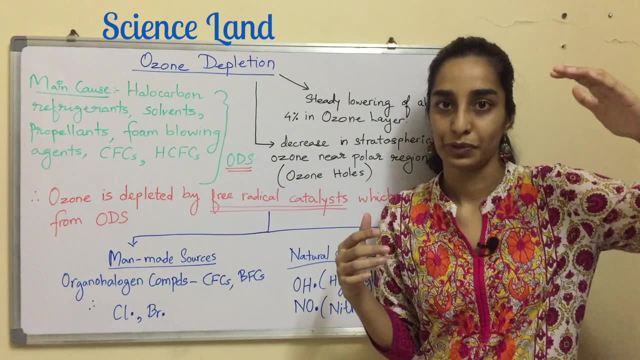 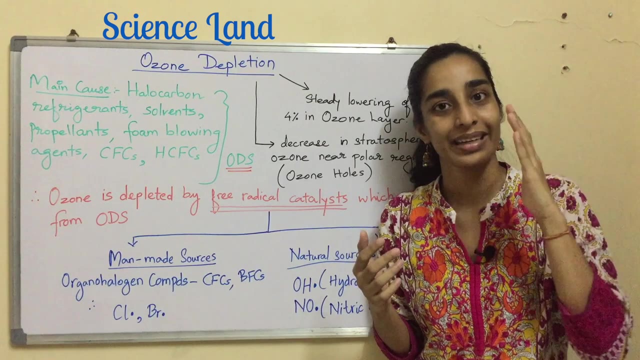 of these organohalogen compounds is CFCs. It is released due to human activity. It will be there in the atmosphere. It will travel to troposphere without any effect. It is very stable, very calm. It will go further, It will go to stratosphere and it will break in the presence. 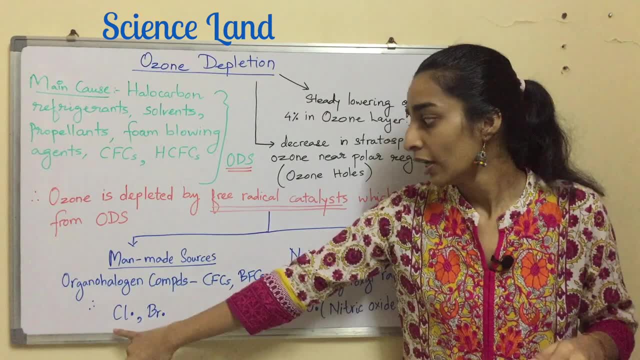 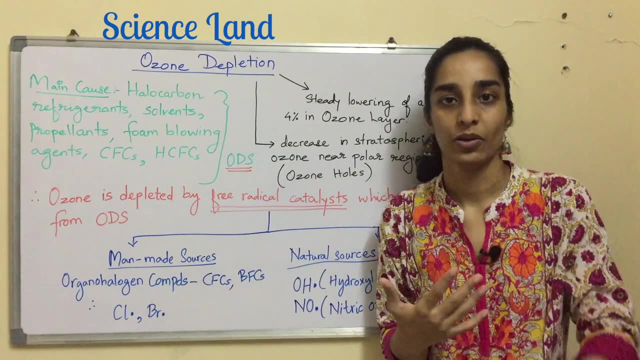 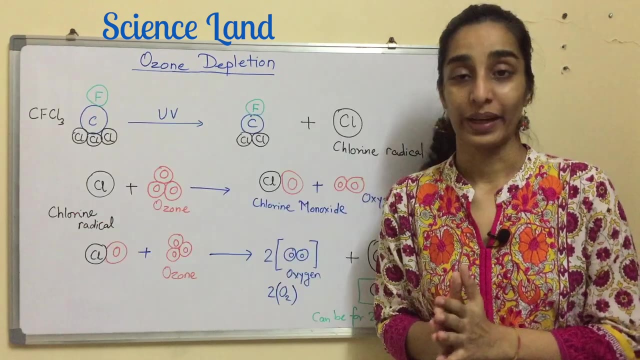 of UV, which will give rise to chlorine radical or bromine radical, depending on the source. It will further break the ozone. Now we will study the mechanism or the reaction of how ozone is broken down. Okay, Now let's study how ozone molecule is actually broken down by free radical. 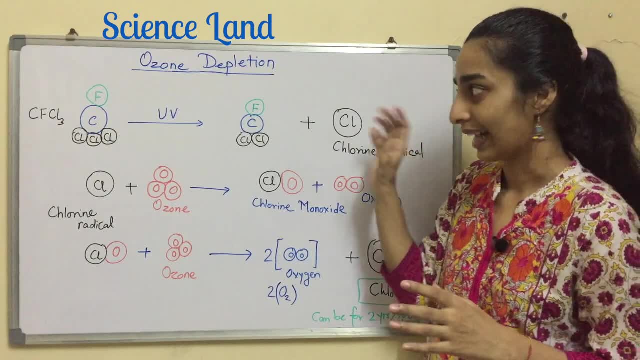 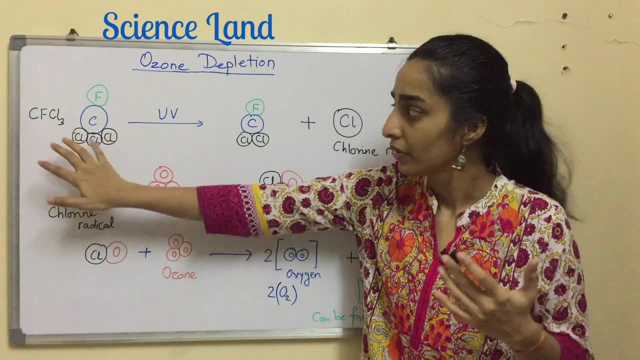 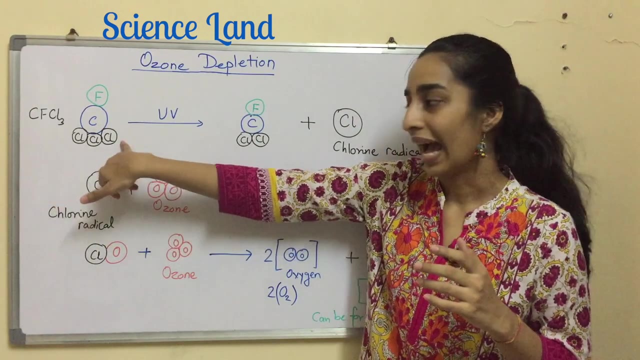 I've written down three reactions, and let's start with the first one. I've taken a starting compound called as CFC- chlorofluorocarbon. The molecular formula for CFC in my case is CFCL3.. Three chlorine atoms, one carbon atom and one fluorine atom. 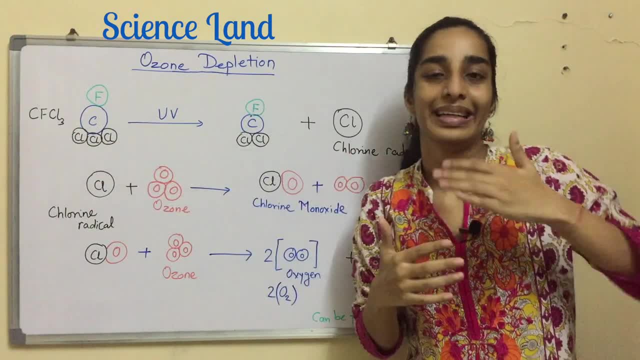 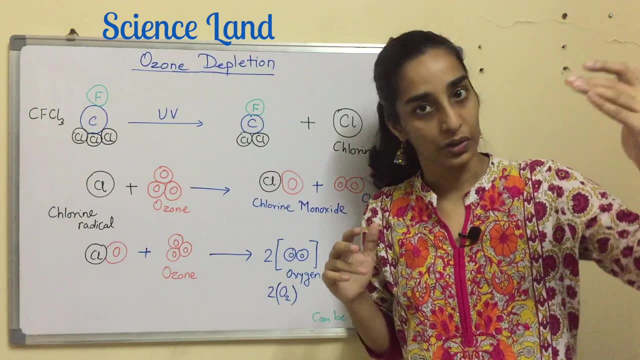 This is the main compound which is released from human activity. It will be not broken down in the troposphere because it is very stable. It will go further in the stratosphere and in presence of UV it will be broken down into two. 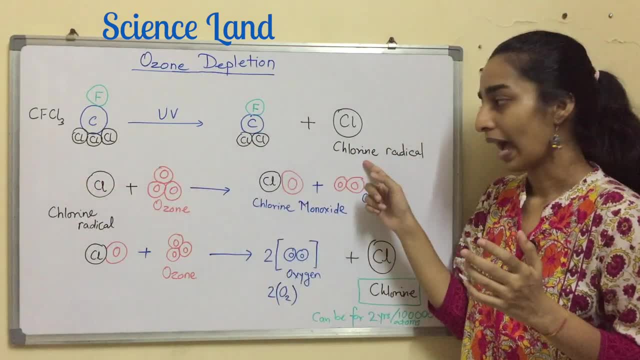 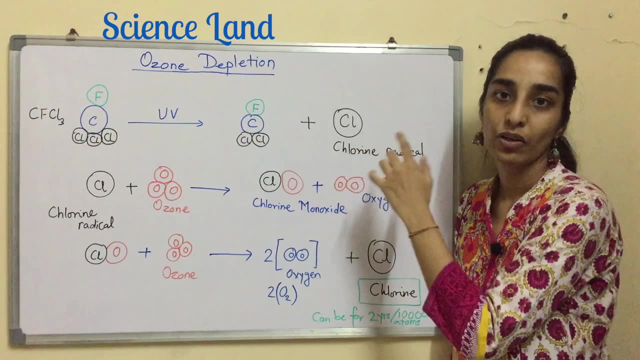 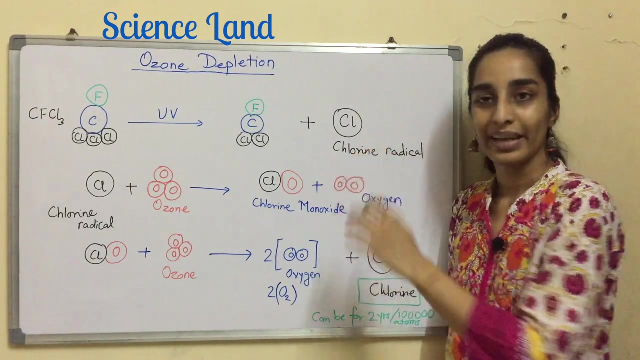 Initially there were three atoms of chlorine. One atom of chlorine is released. The other compound is as it is Now, this free chlorine atom, or free radical, which has a, a free pair of electron with it. it will react with ozone molecule. 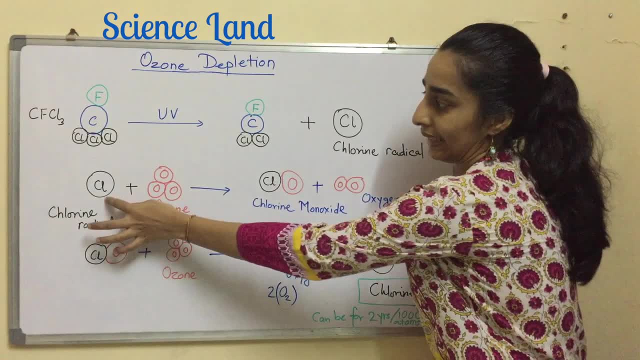 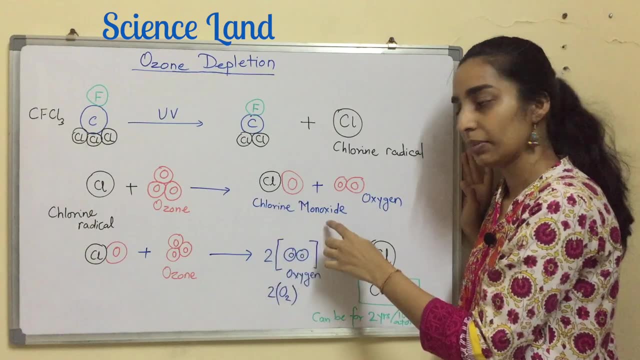 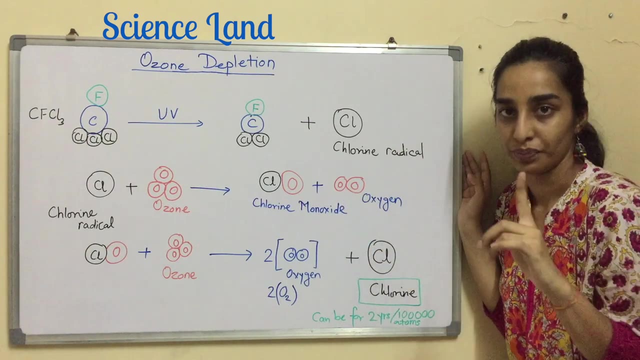 It will break this ozone molecule such that Cl will be attaching to one atom of oxygen, ClO, forming chlorine monoxide, And the other two atoms of O, oxygen, will be forming a molecule of O2.. One molecule of O2.. Further, the reaction doesn't stop here. 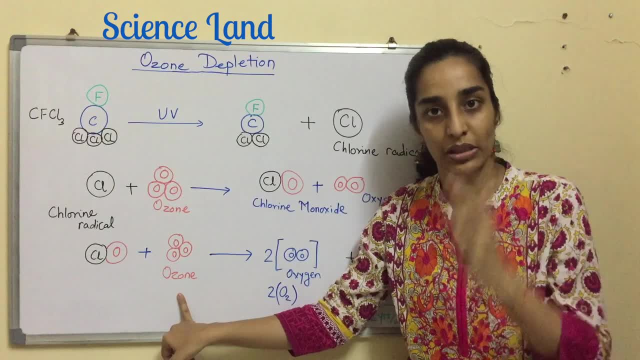 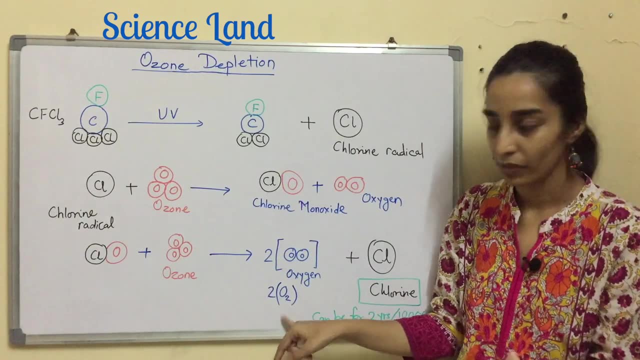 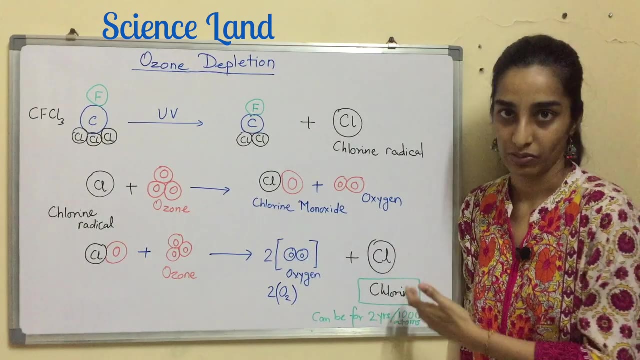 This chlorine monoxide will again destroy another molecule of ozone. It will be forming two products. The first one is stable, which is two molecules of oxygen And one chlorine radical will again be produced. So what you can summarize is one molecule of CFCL3. 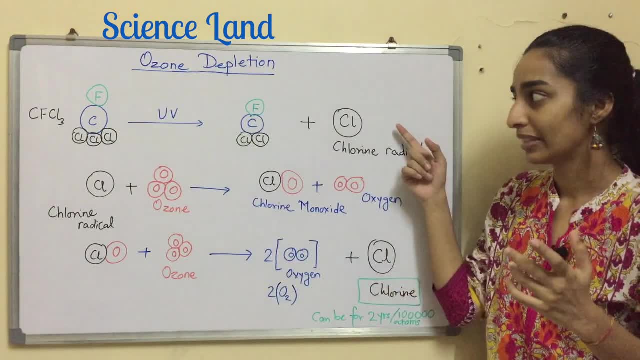 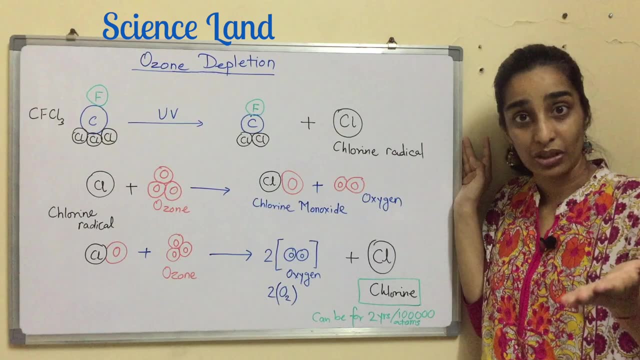 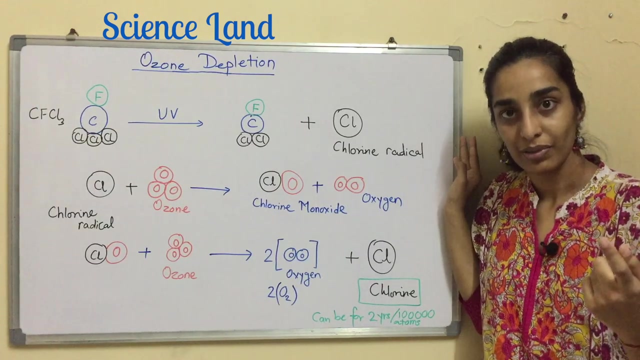 breaks two molecules of ozone by just one release of the chlorine atom, which is there in the atmosphere, Or rather in the stratosphere, for up to two years, And this same radical will keep on breaking ozone molecule till it is actually removed from that cycle. 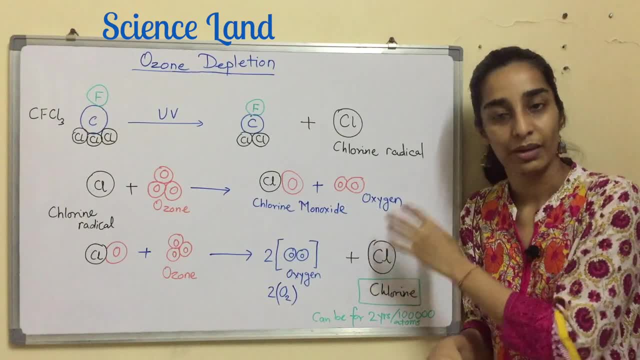 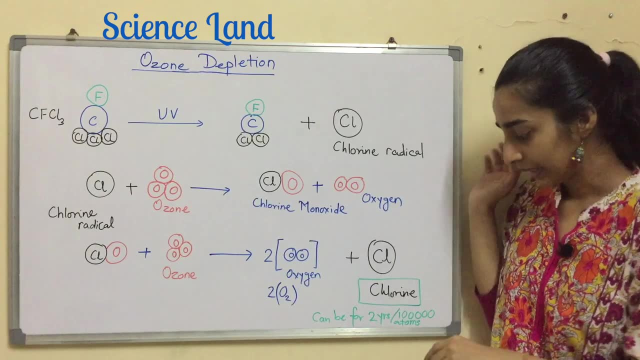 Like, for example, if HCl is formed, this Cl will be used there, So it will be removed from the cycle. But if it is not removed, it will break approximately a lack of ozone molecules, And that's the reason it is known as. 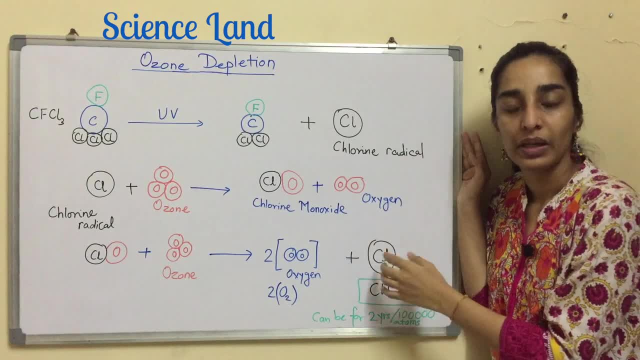 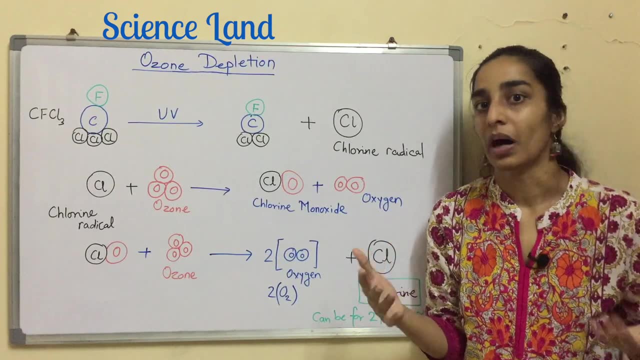 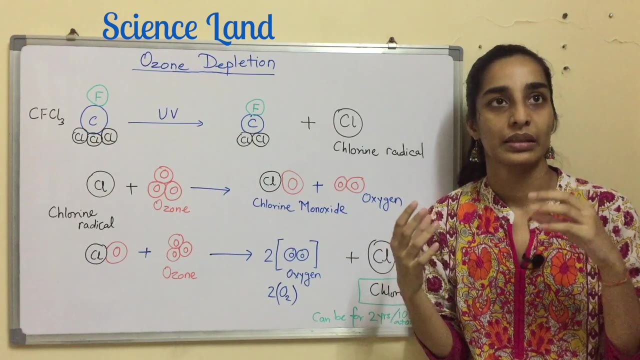 a free radical catalyst. In my example I have only spoken about chlorine, But bromine is even more efficient in breaking down the ozone molecule. Also, there are other two halogens, which are iodine and fluorine. Now, iodine is such a reactive halogen. 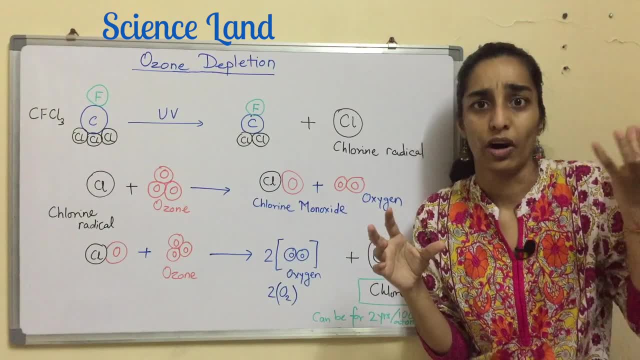 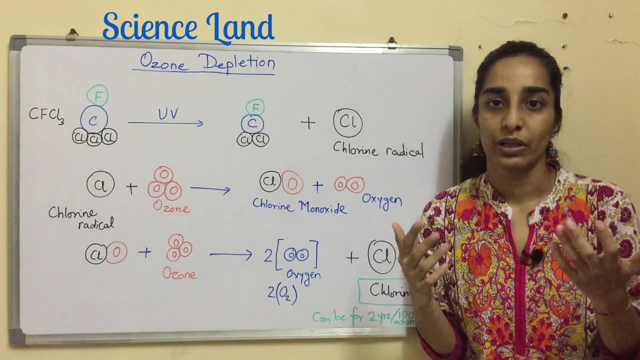 that you know. if iodine is present in any organic compound, it will react immediately in the atmosphere, lower atmosphere- and it won't go further. Fluorine also will react with water and it won't go further. So iodine and fluorine. 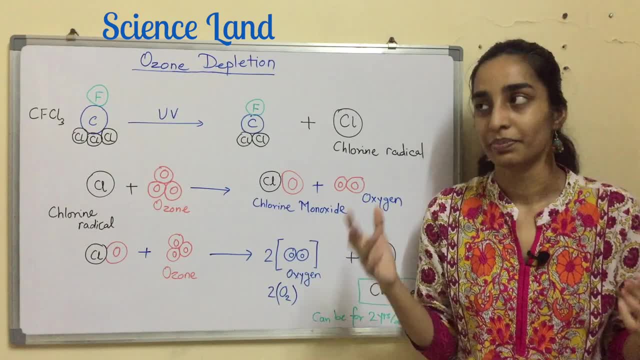 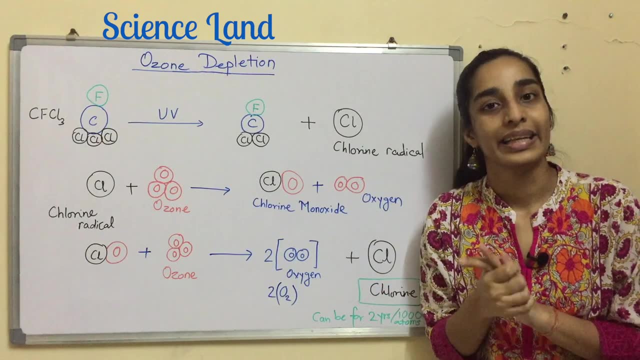 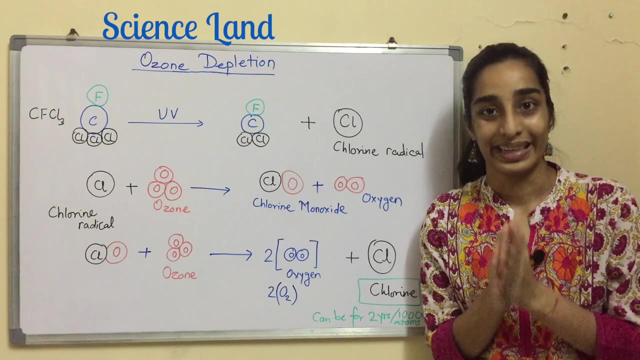 are never a risk to ozone, But bromine and chlorine definitely are risk to ozone. Now to prevent ozone depletion, there is this protocol, which is known as Montreal Protocol. That is to preserve the ozone layer, which we will be talking in our next video.